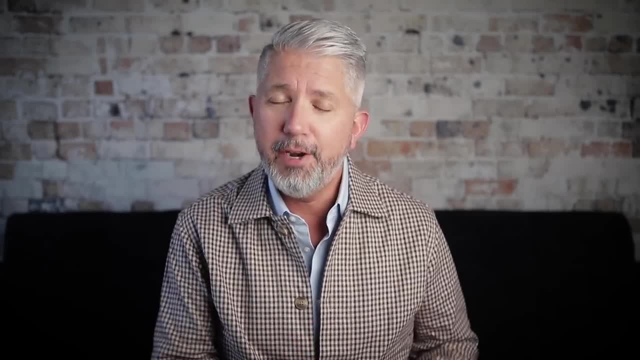 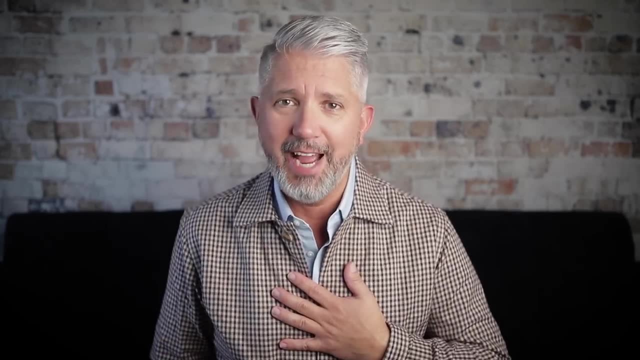 that I'm not too far off from what's considered to be the firm rule And, for the record, you can feel 100% free to throw any colors you want together, if that's your thing, because who am I to stand in your way? However, for the rest of us, there are some things to consider when it 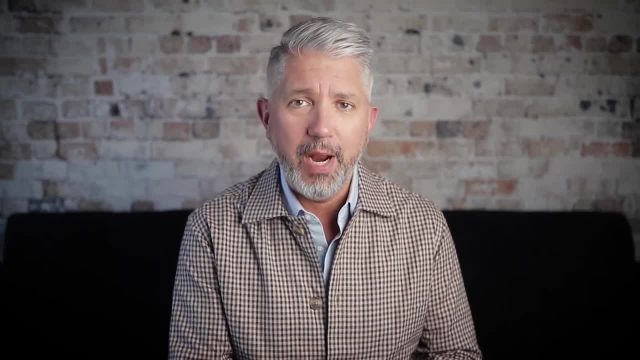 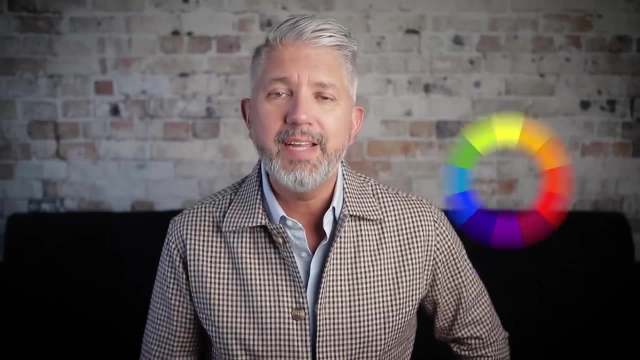 comes to mixing and matching colors. But really quick for the record: yes, you can wear blue and brown together And yes, you can wear black and brown. First of all, take a look at the color wheel. The one I like to use is from Canva and I'll go ahead and link it in the description. 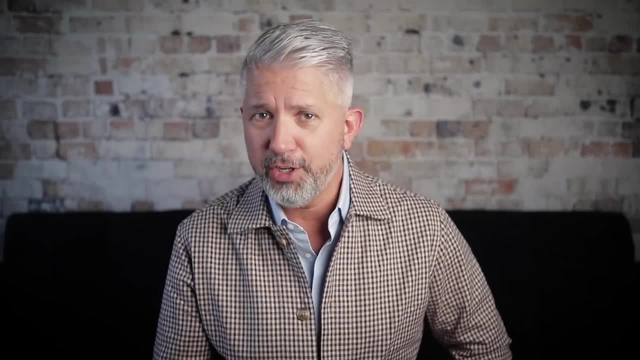 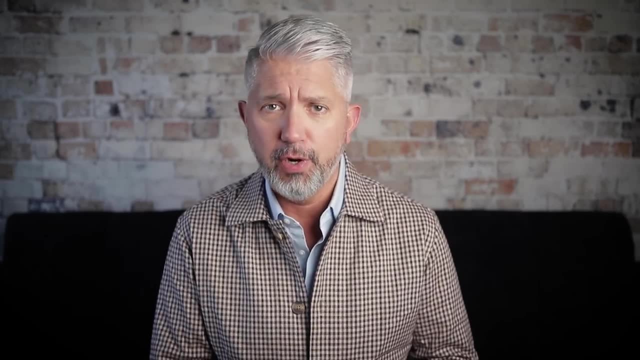 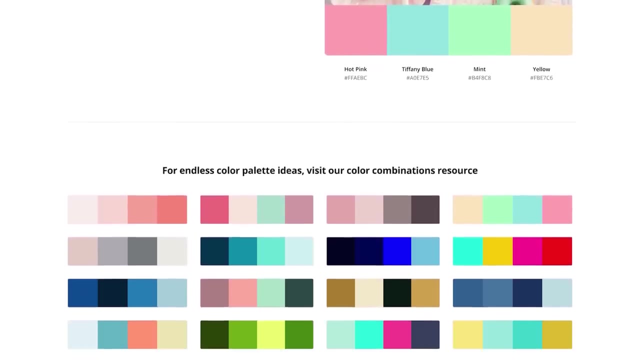 And I'm not suggesting that you print the thing out and hang it in your closet, because no one's going to do that. However, if you're not sure if something goes together, go check it. And I'm also going to link to their color palette generator, which is another very interesting tool to play. 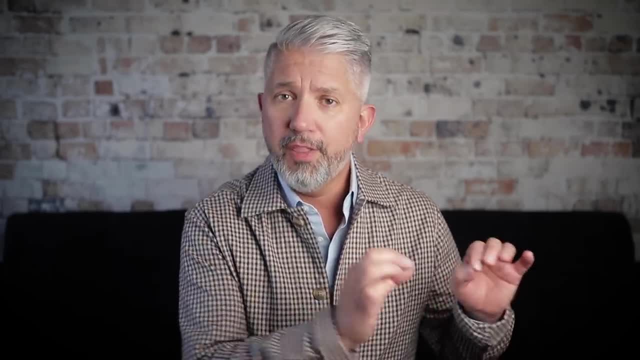 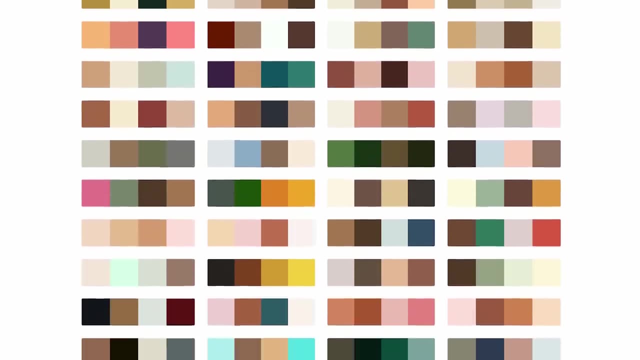 around with. You can look through a ton of examples from what they've put together, or you can type in your own color and see what combinations come up. Then you can use those samples and apply it to your wardrobe. It's definitely worth checking out. So I've seen a lot of conversations pop up. 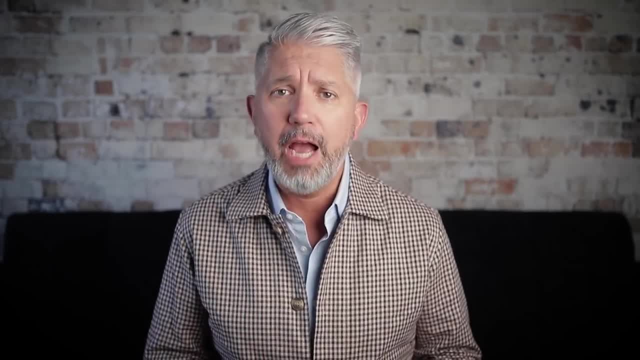 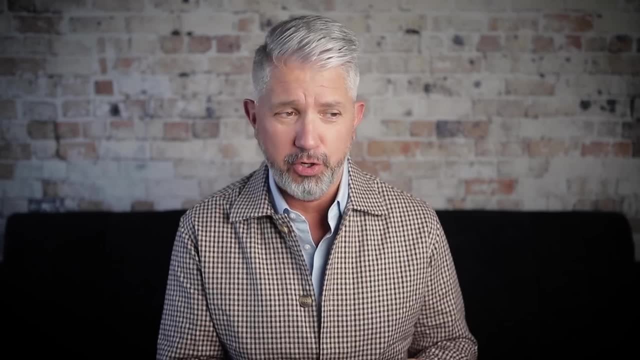 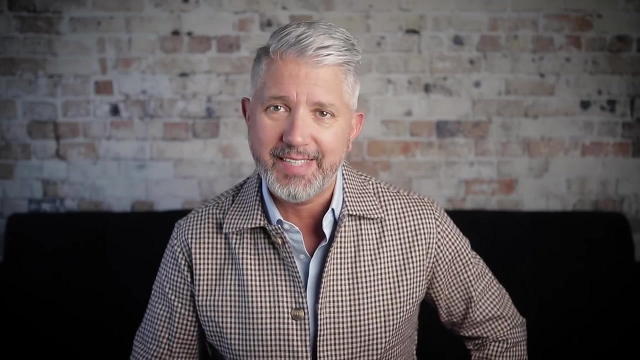 around skin tone and contrast when it comes to how you should dress. So let me take a minute and expand on that. So let's try to group everyone into three categories of personal contrast: low contrast, medium contrast and high contrast. Low contrast guys have very little difference in skin. 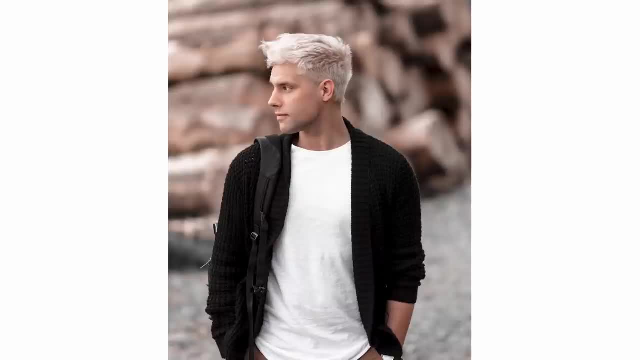 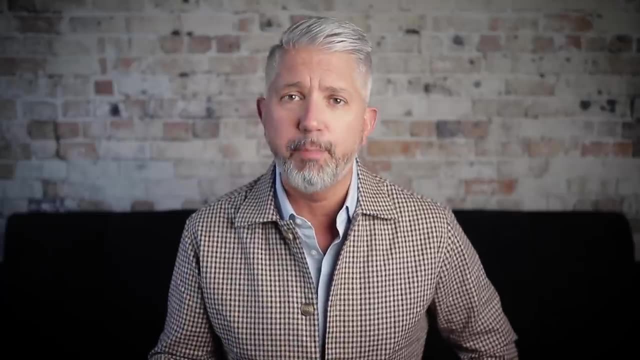 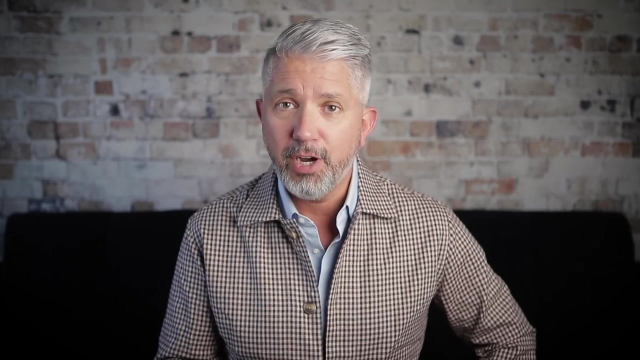 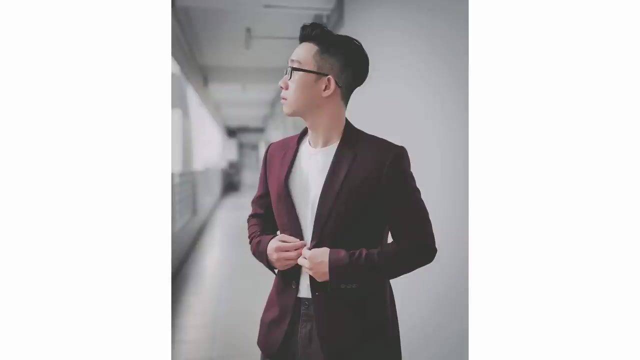 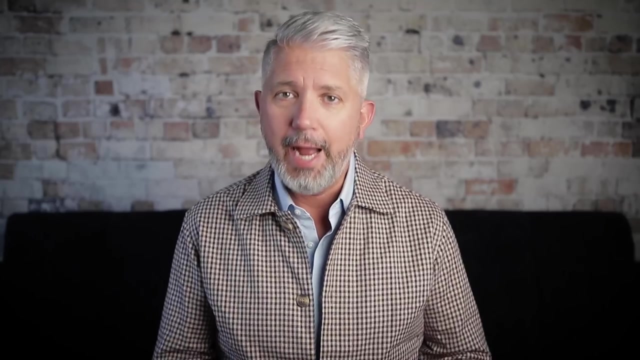 hair and eye color, So think of a light-skinned blonde dude with blue eyes. Medium contrast guys were most of my African-American friends and I think they're going to love this. But if you're a high-contrast guy, wear high-contrast clothing. So think about dark pants with a white shirt. 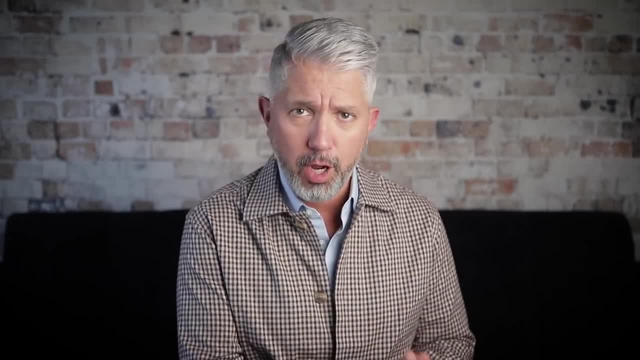 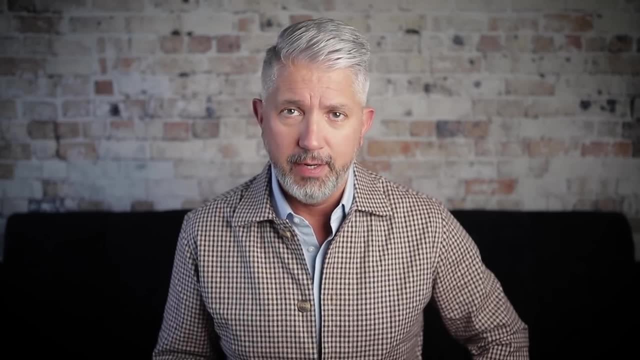 and then a dark-toned jacket. But on the other hand, if you're a low-contrast guy, wear sort of medium tonal items together, right, Think tan chinos, light blue shirt and a light-toned jacket. But if you're so lucky to be a medium-contrast guy, 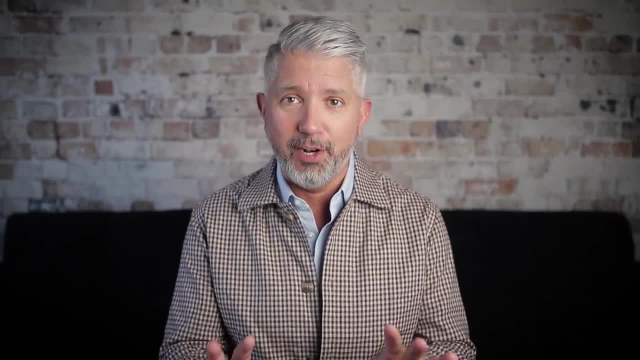 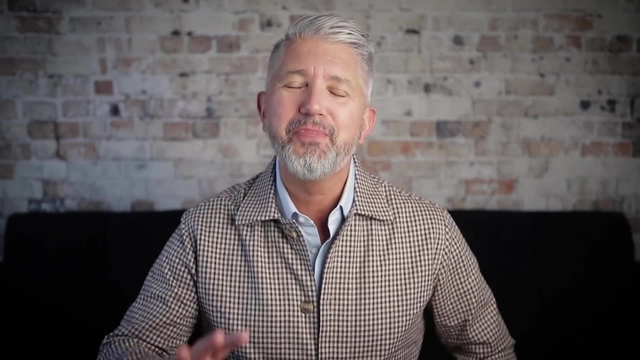 you can practically do whatever you want, because everything is going to look good on you. All levels of contrast look good, and all colors will look good on you. So congratulations, my friend. The bottom line, though, with all of this is to try to mirror the amount of contrast in your face. 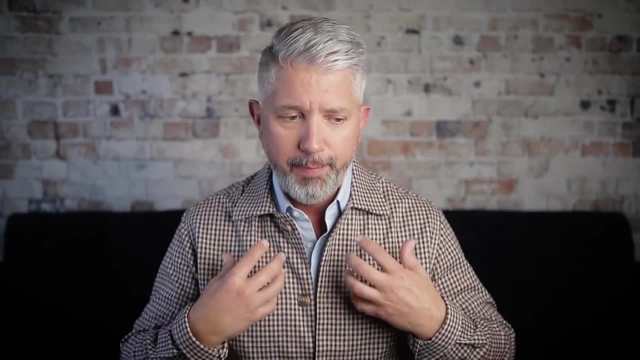 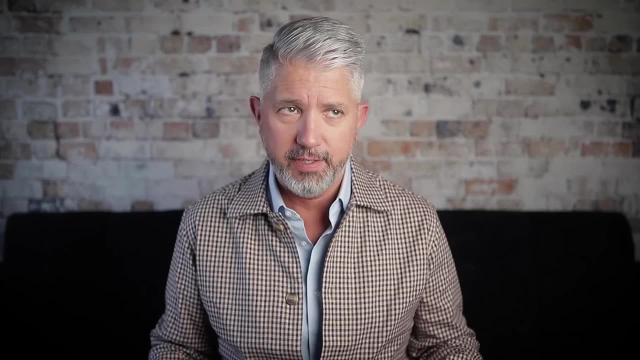 and then apply that to your clothes, especially with your tops, because that's going to be closest to your face. All right, next I want to take a minute and talk about pairing your socks with your everyday outfits And, to keep things very simple, mask the color of your socks to your 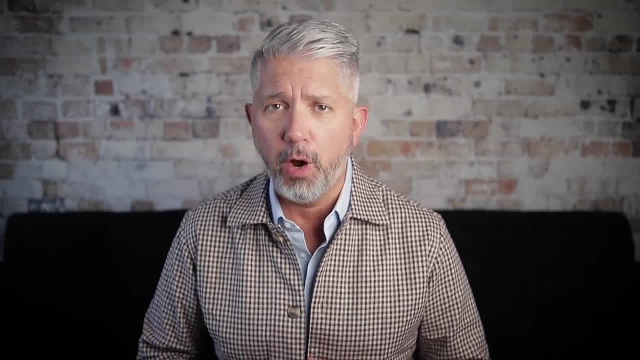 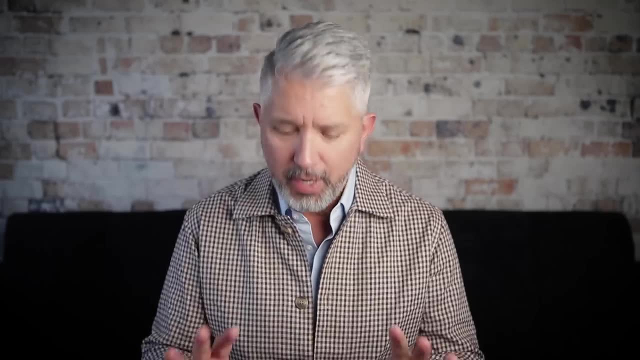 pants color, And it's my opinion, if you have, say, four pair of solid color socks in black and then some shades of blue, brown and gray, you'll be set for just about anything. I've been wearing these socks- from Straight Up Socks- for about the last year and I've been wearing them. 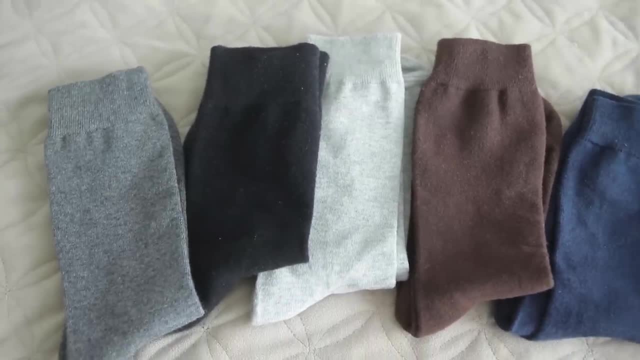 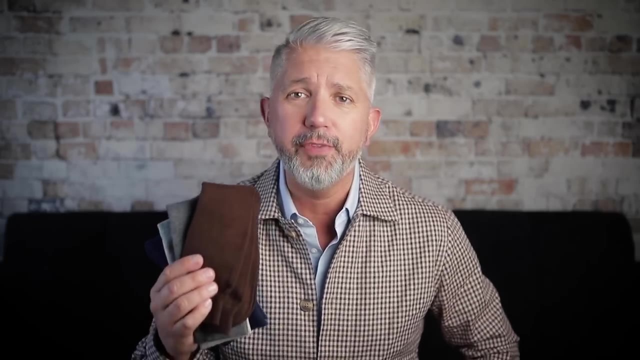 for about a year or so. They use these proprietary silicone strips to keep your socks in place all day long, so you don't have to kind of constantly pull them up all the time, And the small silicone strips hold the sock in place instead of relying on tightness and squeezing your legs to death. 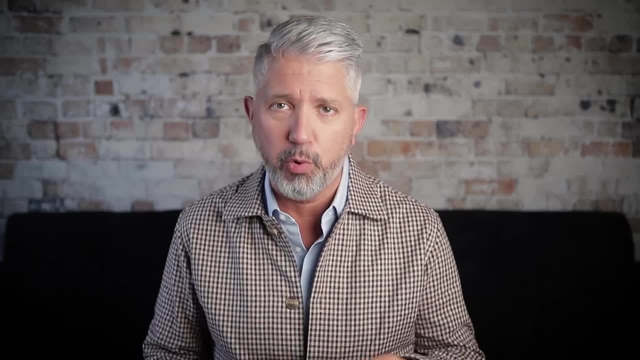 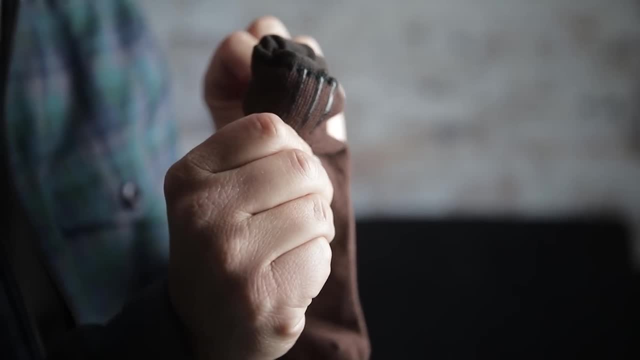 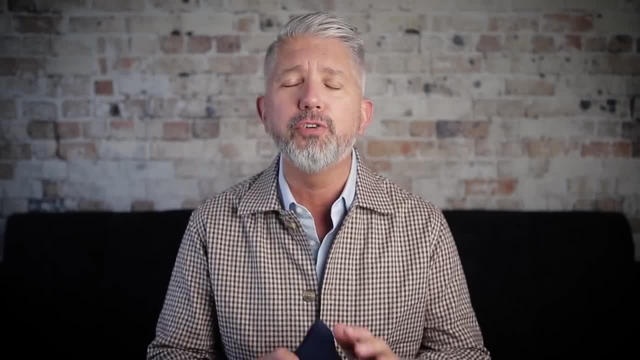 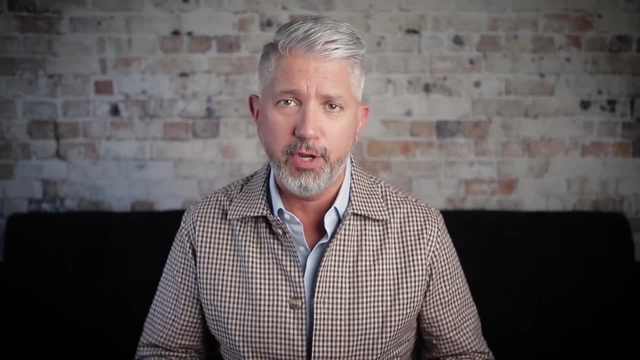 link down in the description and enter the code below for a special offer on your total order. Thanks again to Straight Up Socks for sponsoring this video. Okay, now let's talk about achromatic outfit combinations. So these are going to be your black, gray, white and, of course, all the 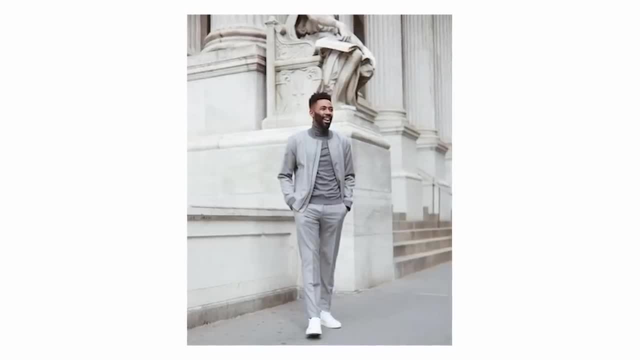 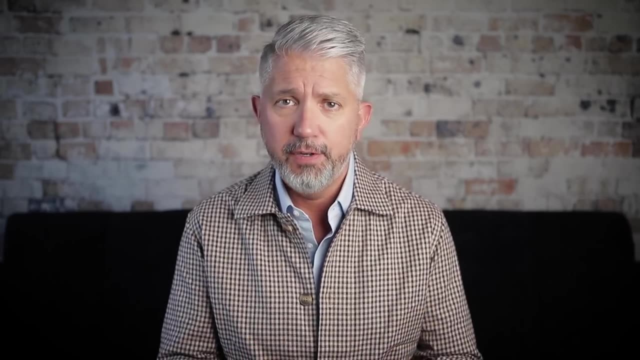 shades of gray in between, So you can go dark gray pants with a light gray shirt and then a medium gray jacket with white or black shoes. Basically, it's totally safe to combine different shades of gray, black and white together in the same outfit. Okay, now let's get into colors, for. 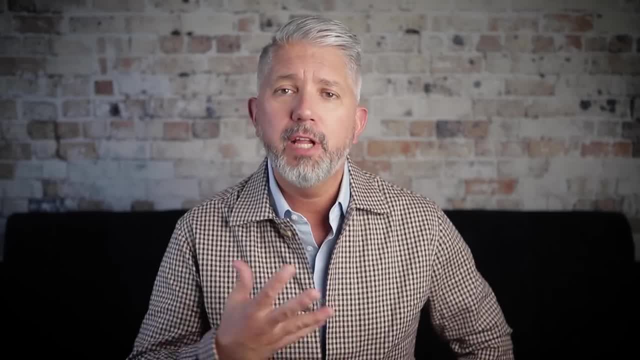 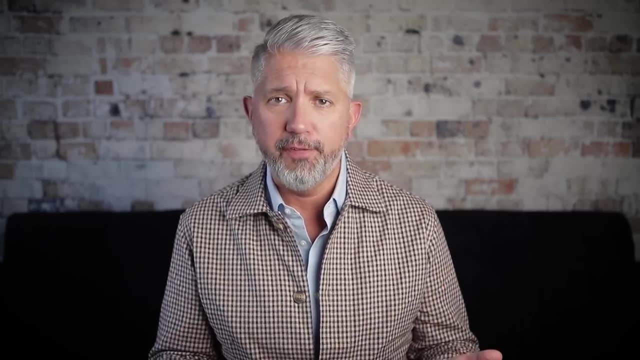 a little bit right. So we talked about skin tone a little bit ago, So let me mention another aspect of that that can help you choose colors that are best for you. So all of us have a certain skin tone that falls somewhere within sort of a warm to cool skin tone. So if you're looking for a 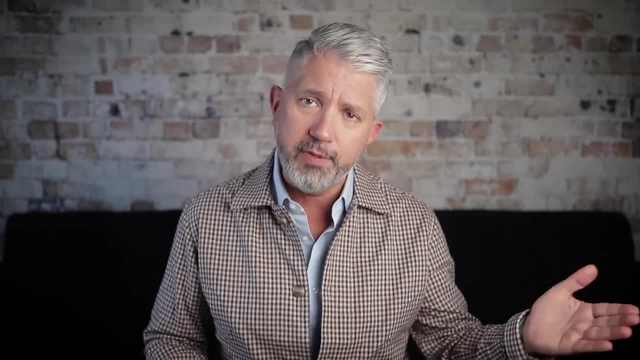 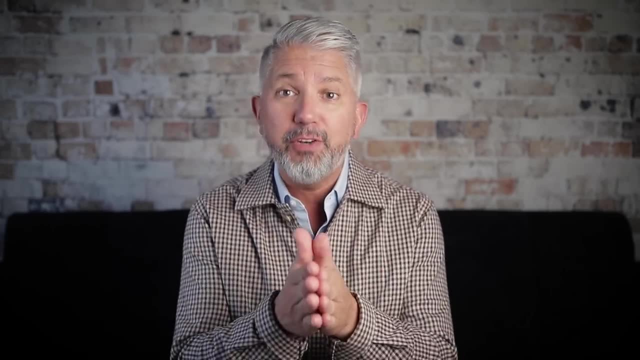 cool scale and if you have darker skin you're probably going to fall towards the warm side of the scale. People with lighter skin tones are kind of where things get a little more complicated, because some people can fall right towards the middle. But if you want to check for yourself, 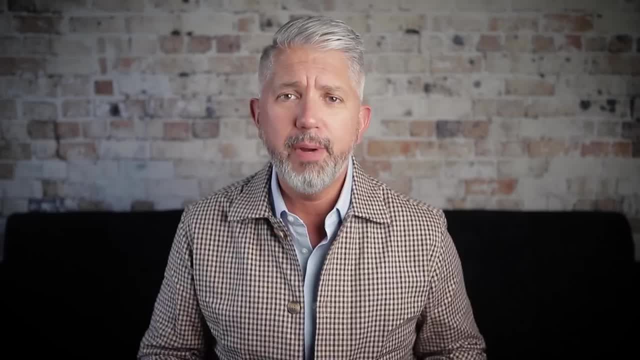 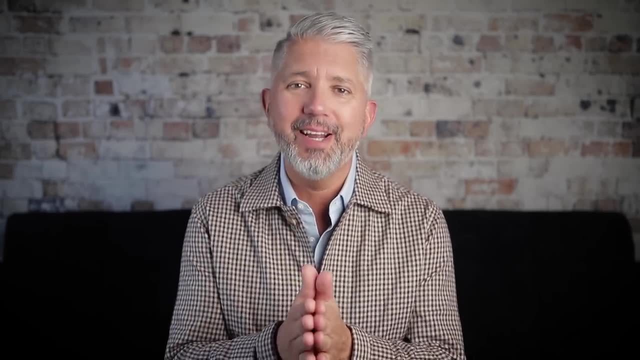 look at the veins in your wrist. If they appear blue, you probably have a cooler skin tone. If they look more green, you probably have a warmer skin tone, And if you can't tell, you're probably somewhere in the middle. Also, think about how your skin reacts to sun exposure. If your skin gets red, 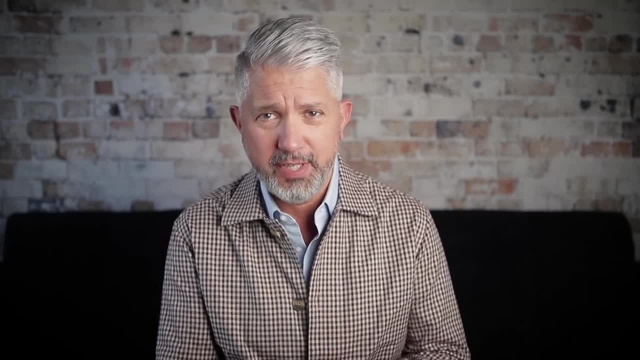 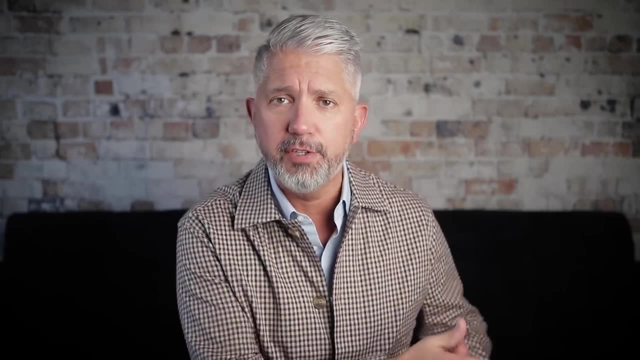 and you tend to burn pretty easily. you're probably going to have a lot of sun exposure And if you tan easily when you're in the sun, you probably have a cooler skin tone. But if you tan easily, you probably have a warmer skin tone. So, knowing this, along with the contrast we just talked about, 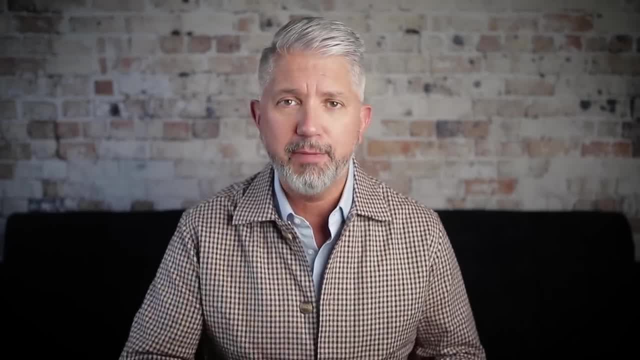 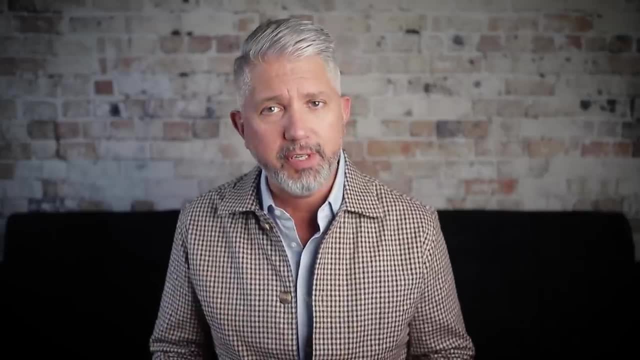 earlier can help you choose colors that look best on you. Let me explain. People with cooler skin tones tend to look best in colors that are on the cooler side of the spectrum, And people with warmer skin tones look best in colors on the warmer side. And a couple words of caution. if 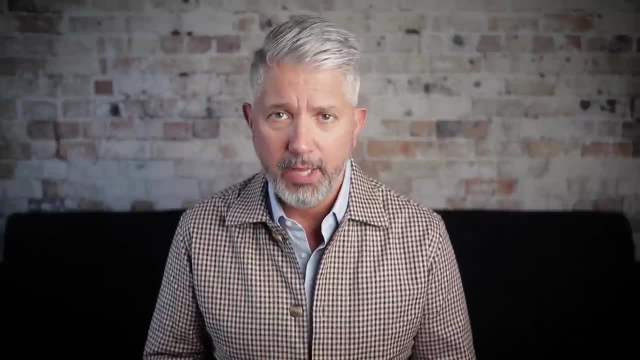 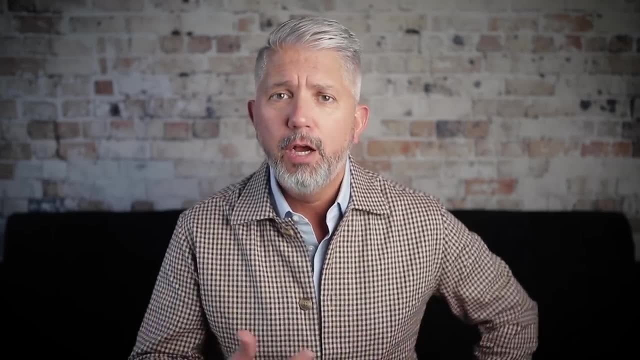 you have cooler skin tone, Avoid bright yellow, red and orange colors, because that will clash with your skin tone. Also, if you're on the pale side, avoid light pastels close to your face, like light pink and light blue. These pastels can kind. 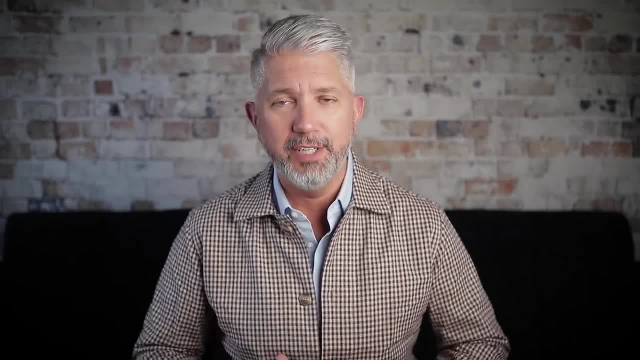 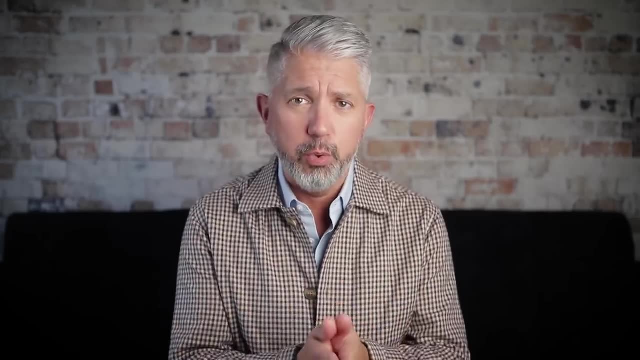 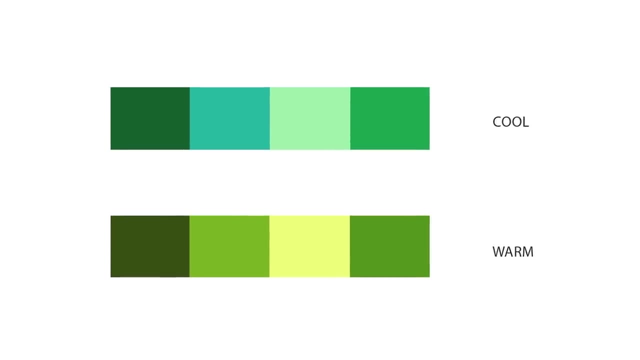 of make you look washed out because they're almost too close to your actual skin tone. Okay, here's a couple visual examples for you, showing the same color, but also the subtle differences between warm and cool shades of that color, And these might not be perfect, but you can get the idea. So here's a cool green and a warm green. 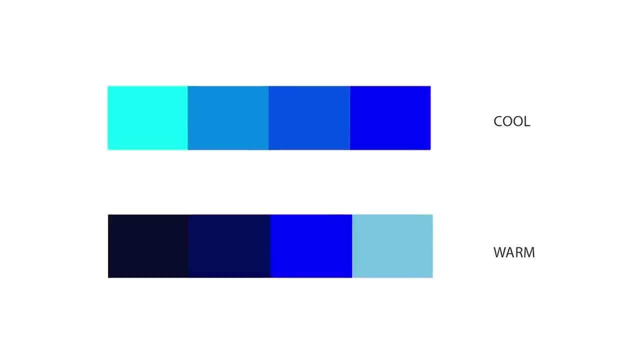 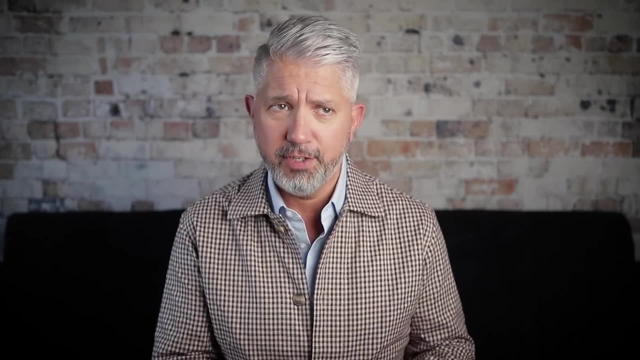 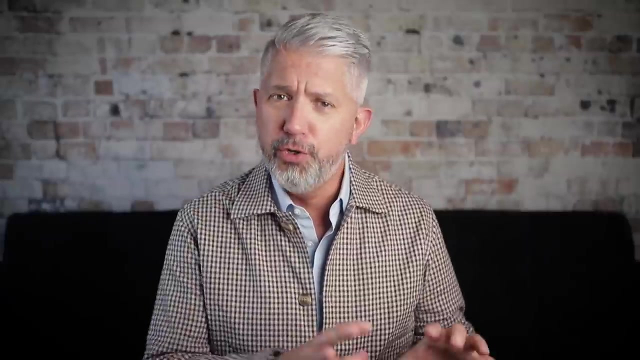 Here's a cool blue and a warmer blue. Here's a cool red and a warmer red. So it's not like you can't wear specific colors right. Just be more aware of the subtle undertones of that specific color to make sure it'll look best on you. Okay, let's talk neutrals for a.